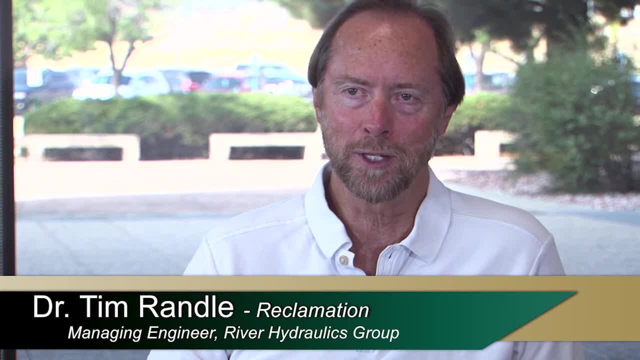 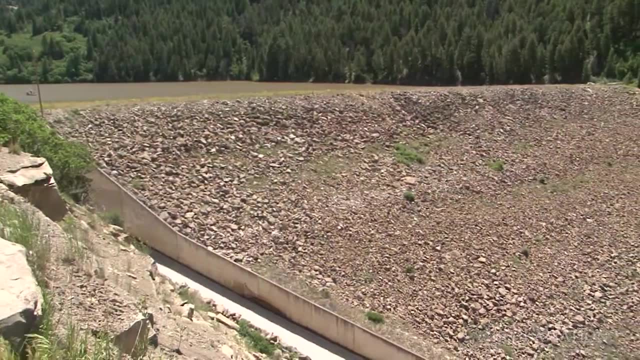 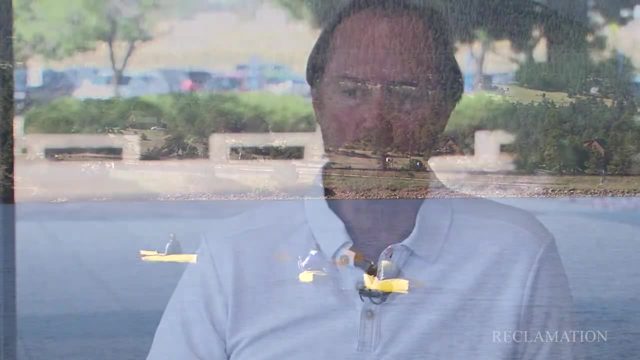 Sedimentation is affecting the project benefits for the nation's reservoirs. It's by filling up these reservoirs gradually over time, reducing the storage capacity, impairing outlets, impairing boat ramps, marinas, impairing space for recreation, And we need to look at ways to better manage sediment over the future, more sustainably. 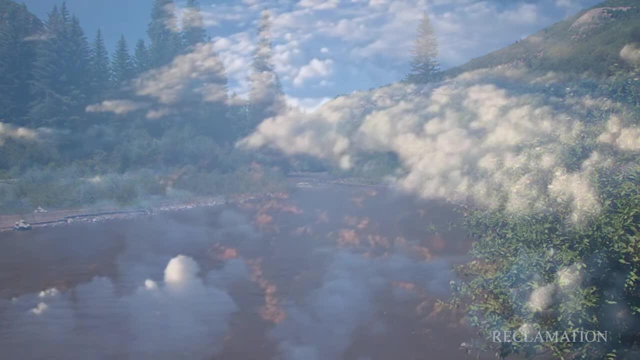 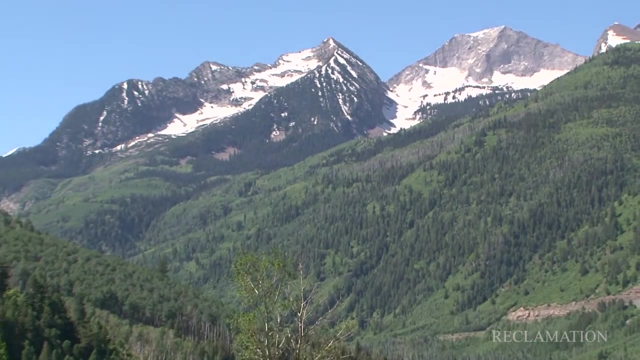 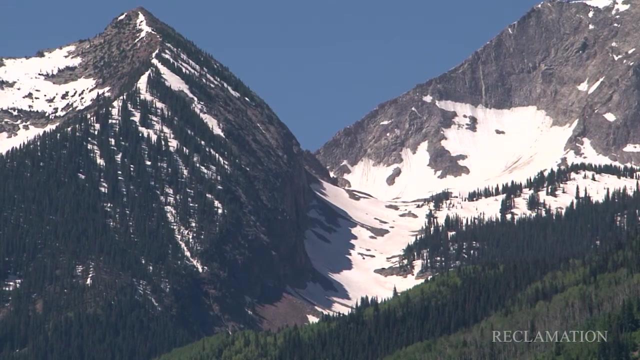 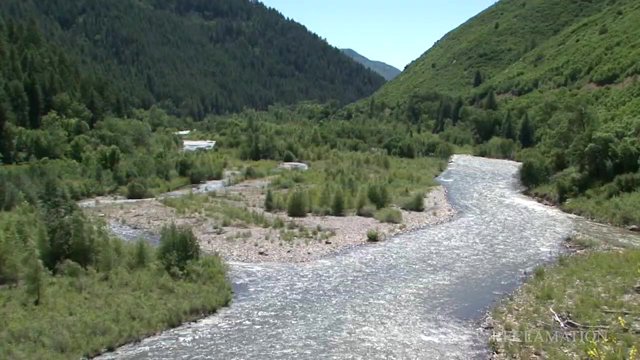 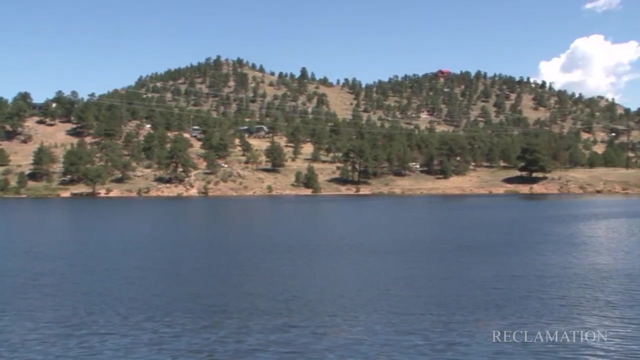 The sedimentation rate that we see in the reservoirs is driven by: one, the weather patterns. two, the geography associated with that reservoir. When we have reservoirs in areas that have high rainfall, steep mountain valleys, high amount of sediment available to come run off the watershed, all of those things contribute to high loads that can result in accelerated loss of storage volume. 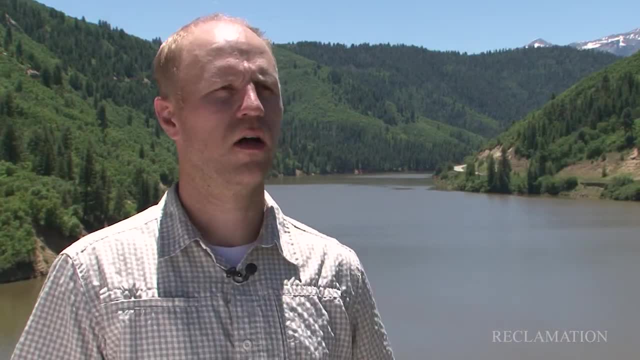 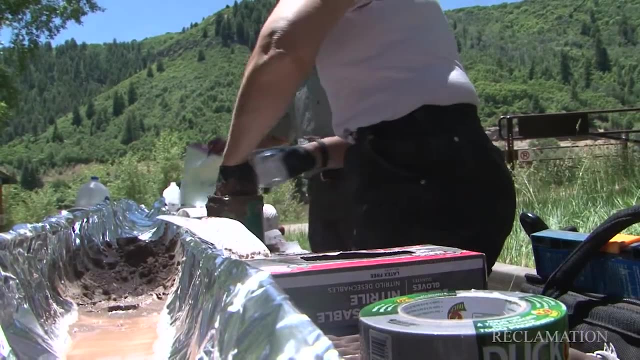 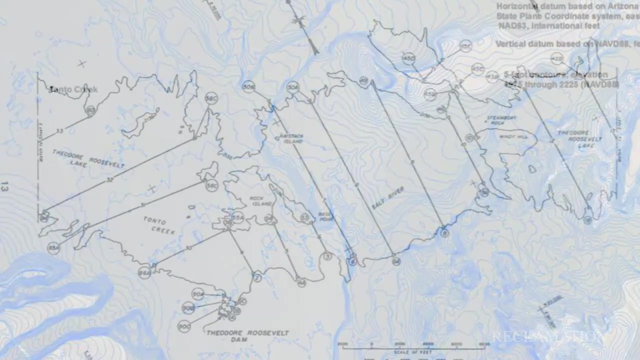 Current methods measure a reservoir's sedimentation are in two ways. The first is direct measurements, where you have a boat with a depth sounder and GPS mounted to it and you map the bottom of the reservoir And then you compare that map that you've created to an older survey. 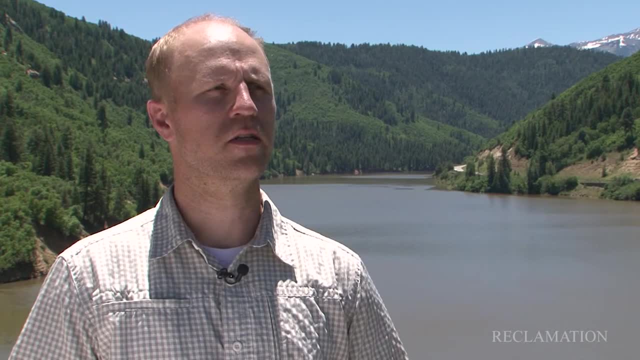 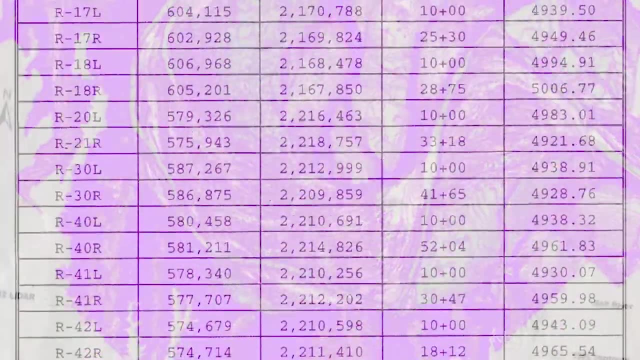 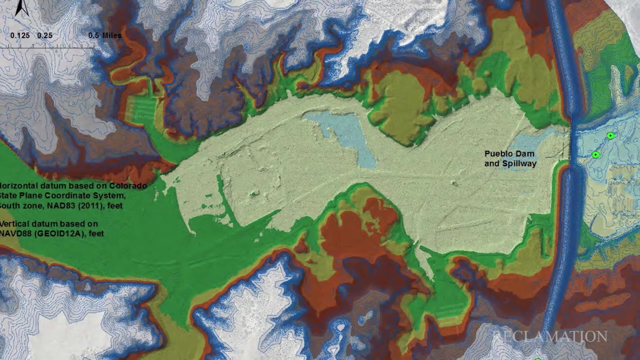 The second way to measure reservoir sedimentation is indirectly, where you're using modeling techniques- whether it's an empirical type of model or an analytical or even physical model- To indirectly estimate the amount of sediment accumulation in a reservoir. One of the biggest limitations is just our capacity to do it. 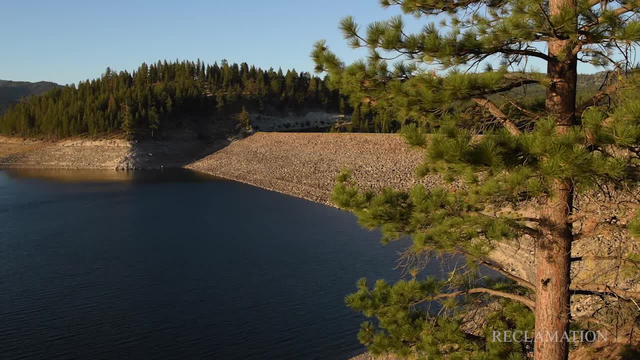 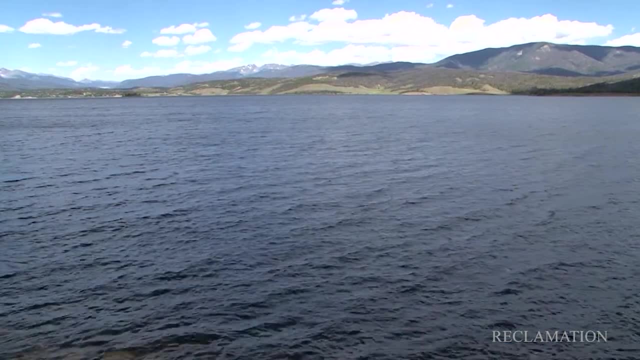 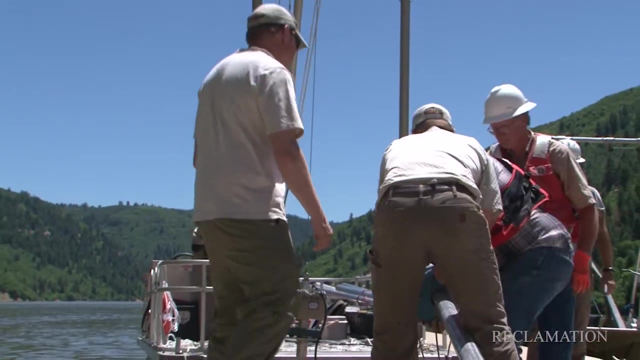 There's 300, some reservoirs and reclamations inventory, many more when you look at the whole federal sector and private as well. And there just haven't been that many surveys, largely due to cost. These traditional methods require personnel on the ground to do that and to get to these remote areas. 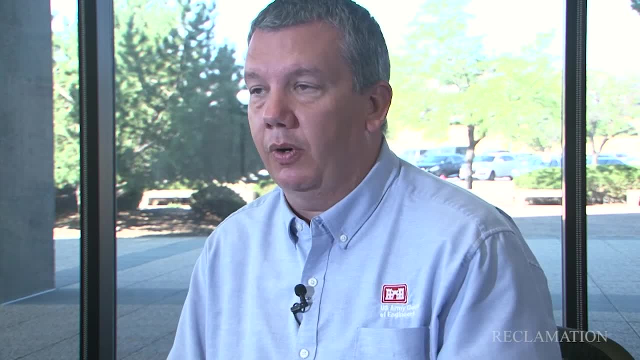 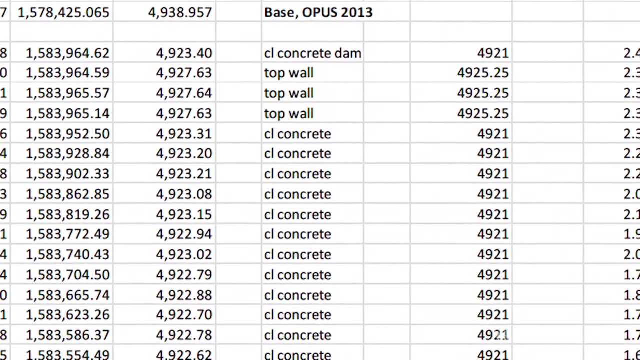 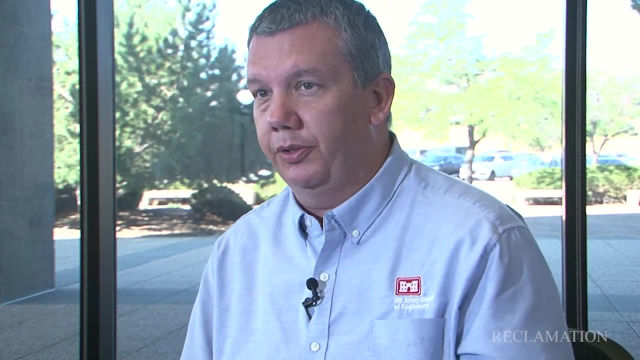 And as budgets are limited and we try and be the best stewards of the resources we can, we have to make trade-offs For indirect methods. the limitations are simply that our estimate is based on the quality of the data that's available to either do numerical modeling or watershed runoff estimates.